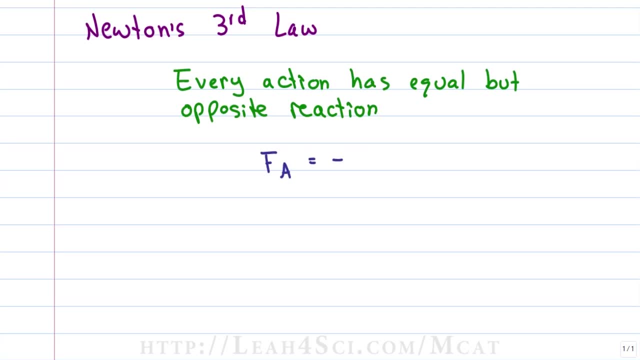 Mathematically, we write this as: F of A is equal to negative F of B, and what this is telling us is that the force of object A acting on object B is equal to negative, meaning the opposite force of object B acting on A. There's no sign in front of F of A, which implies that. 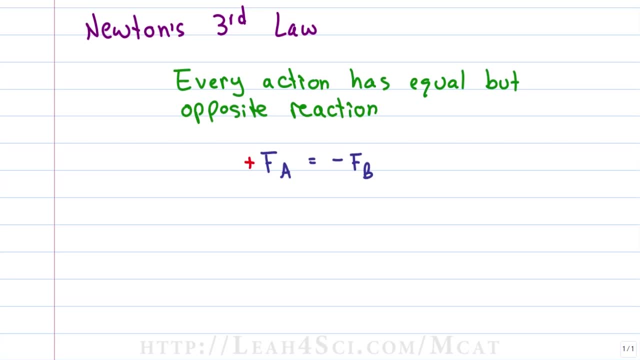 it's positive and this simply tells us the direction. If the force of A to B is right, then B to A is left. If A to B is up, then B to A is down. It's simply equal, but opposite. Think back to the block we used in previous examples. We showed a stationary block with 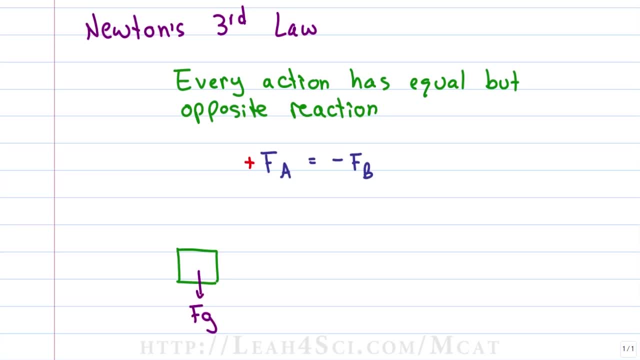 two forces acting on it. We showed a downward force of gravity and an upward FN or normal force. You can think: hey, if F of N is up and F of G is down and they happen to cancel each other, meaning the sum of the forces in the Y direction are equal to zero. such, 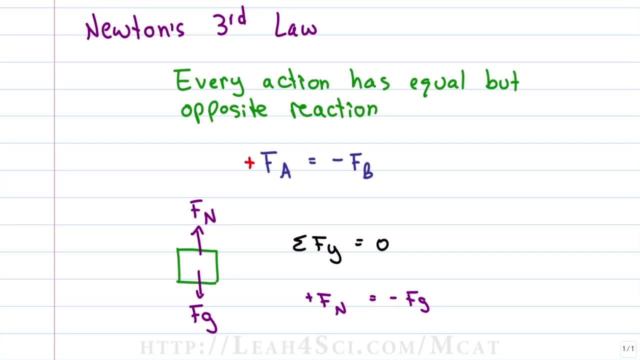 that F of N positive is equal to F of G negative. This is not the case. This is not Newton's third law, because both of these forces are acting on the block. This would be F of N on the block and F of G on the block as well. Newton's third law tells: 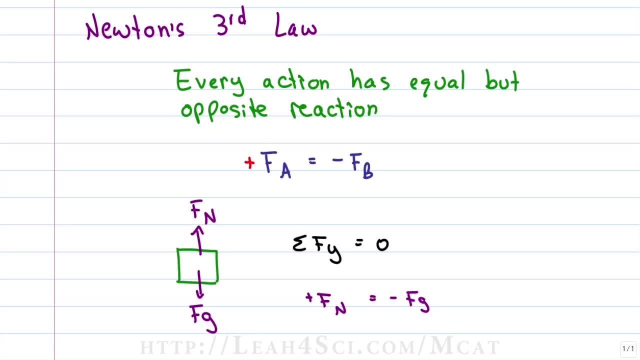 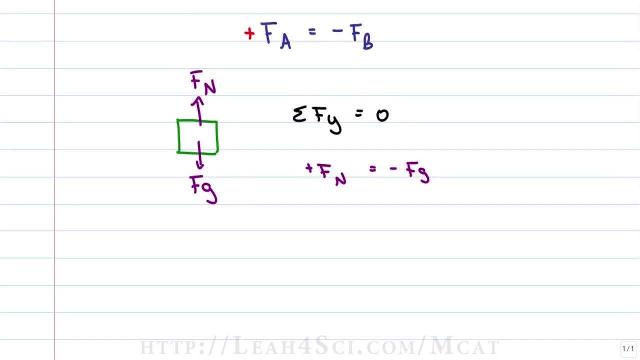 us that the two forces relate to two objects acting on each other. So if we look at the block again, if the force of gravity is a downward pull, then what we're really seeing here is the force of earth on the block. So this is the force of gravity. 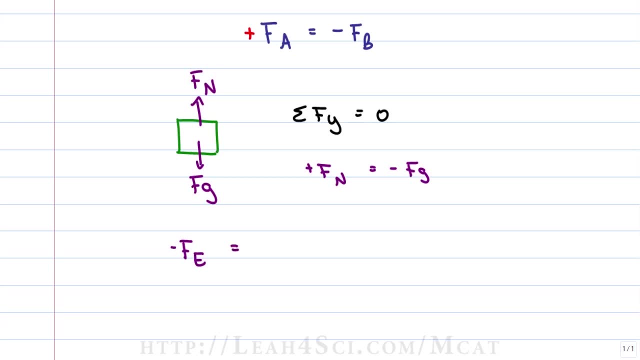 So the force of gravity is a downward pull of the earth on the block. Because earth is pulling down on the block. earth is pulling down on the block. that's negative, That is equal and opposite to the force of the block on earth. Earth is pulling down on the block. 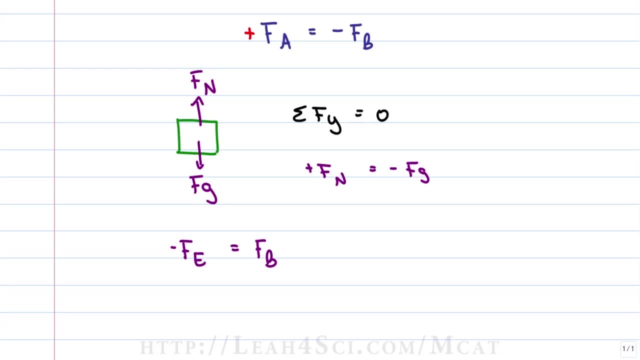 and the block is pulling back up on earth with an equal but opposite force Because the block is tiny compared to earth. earth putting a little bit of force onto the block block is negligible, so earth is not going to move just because of a little object sitting. 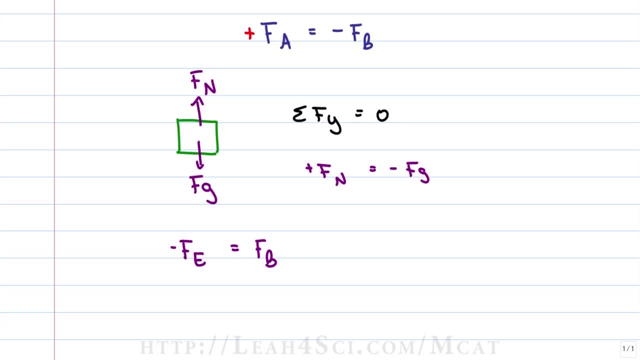 on it, But mathematically the force is exactly the same. Let's put this into numbers and let's say that the block has a mass that is equal to 10 grams. If we want to figure out the force of earth on the block or the block on earth, we just 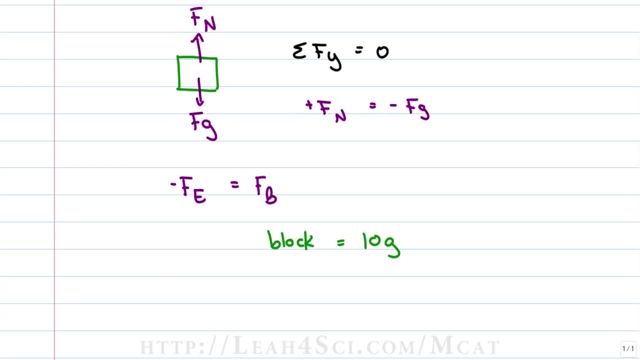 have to solve for one and then simply choose a direction. How do we figure this out? Well, force can imply weight, right? Weight is simply the force of gravity, which is mass times, the acceleration of gravity, MA, or simply MG. Remember that this has to be in kilograms, because force is measured in newtons, which 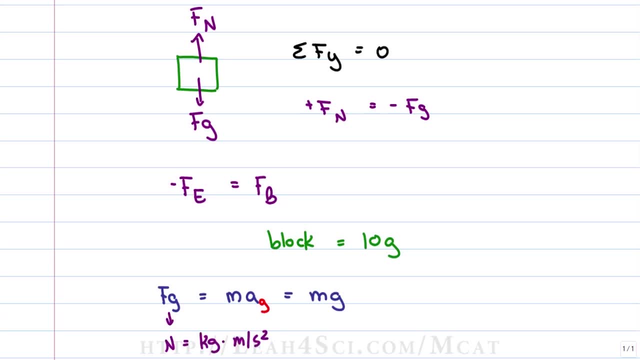 is kilogram times meter. per second squared mass times, acceleration. Plugging in the values, we have 10 grams, which we quickly convert to kilogram by moving the decimal back three spaces. remember: kilogram is 1000 grams. That means we have 0.01 kilograms. 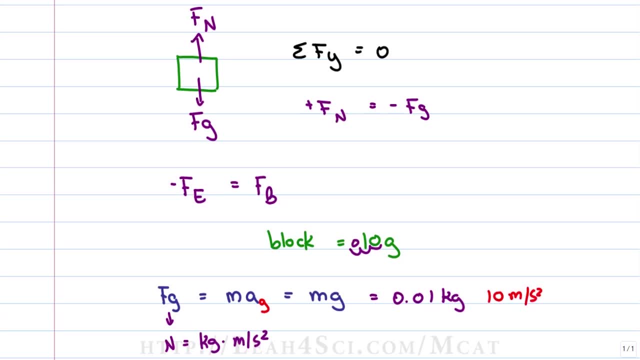 So we have the force, which is 0.01, into 0.01 newtons, which is 0.01 kilograms times the acceleration of gravity. So we can do this noggin for the first time. So we take the force which is 0.01 kilograms times 10 meters per second squared, which is 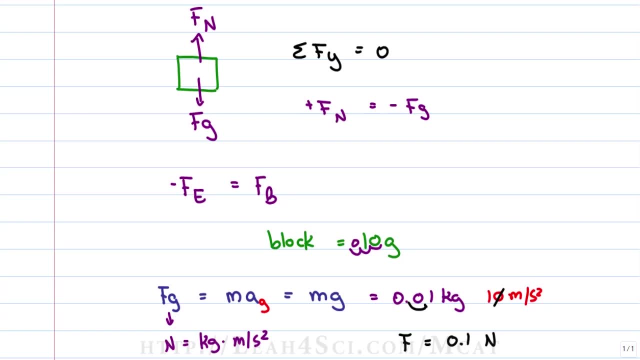 the number to memorize for acceleration on the MCAT. and then we multiply using the decimal trick. 10 has one zero, which means one decimal to the left, and so we move this one to the right, the block downward, and the block is exerting a pull of 0.1 Newtons on Earth in the upward. 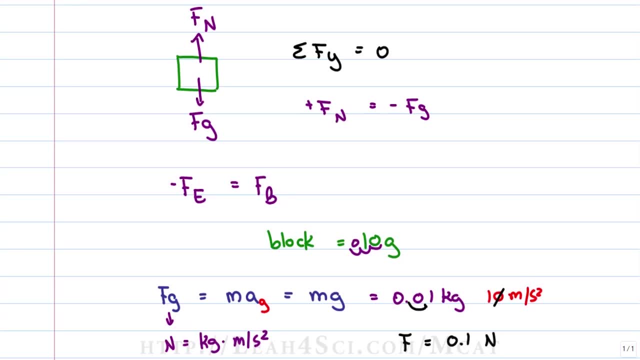 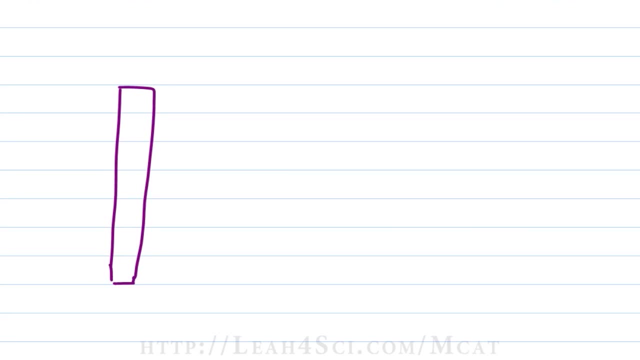 direction. I realize this is where many students get confused, so let's look at another example. Imagine there is a giant brick wall and it's not moving. This brick wall is in total equilibrium. We have the force of gravity. the weight of the wall is perfectly countered by the normal. 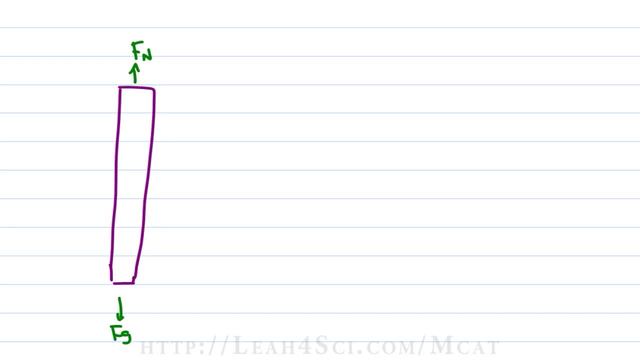 force, and there are no forces in the X direction to push the wall to the right or to the left. And now you come along and you decide you're going to push the wall. So you hold your palm out and you give a slight little tap onto the wall. 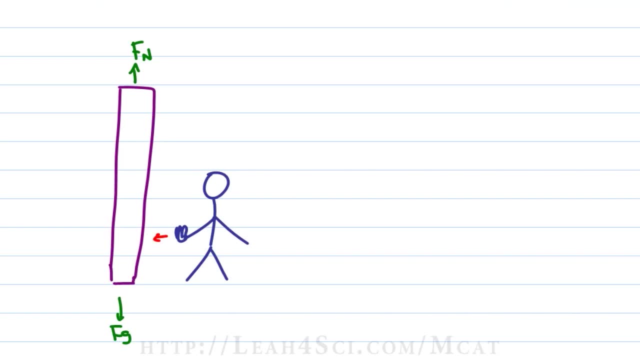 Assuming you're not Superman and you're not strong enough to just knock over a giant wall with a single tap, we're gonna say that your force on the wall is small and we'll call that negative because you're pushing to the left. That's the force of the person. 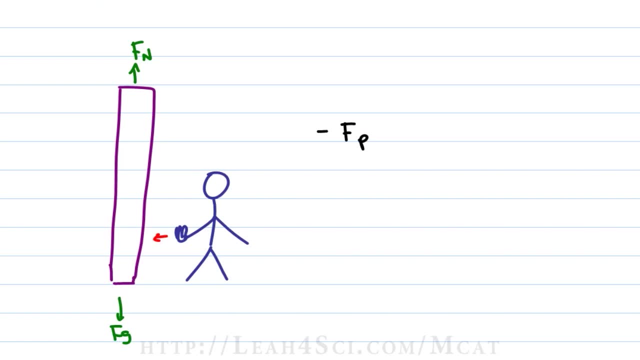 But when you tap the wall, the wall doesn't move. Now, if the wall did not exert a force back onto your hand, then the net force on the wall would be that tiny little tap and logically the wall should topple over. But the fact that the wall does not topple over when you give it a slight tap implies 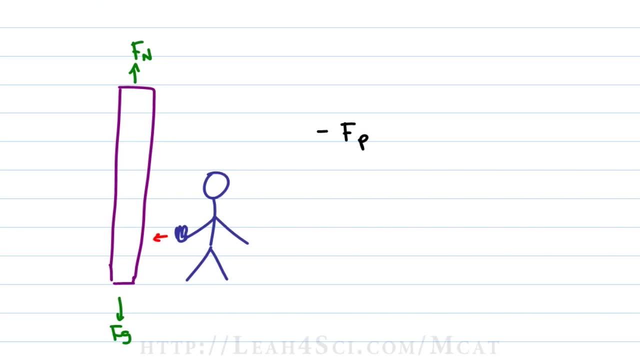 that there is a force countering your tap and that force keeps the wall at equilibrium and keeps it from falling over. So the negative force on the wall is countering your tap. So the negative force on the wall is countering your tap. The negative force should be equal to opposite the force of the wall. So you throw it to the left, Even more so when the wall pushes back beside of the table by theили force of the person, which is, in this case, equal to opposite the force of the wall if you push with 1 newton. 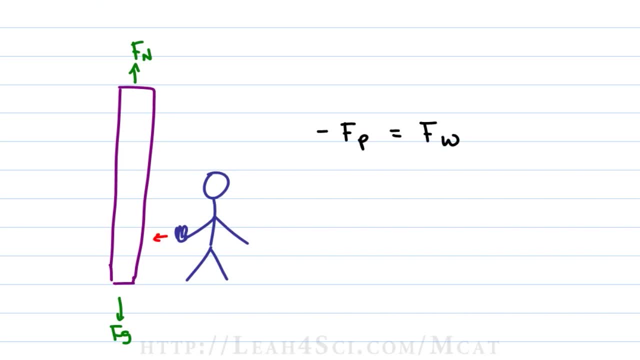 the wall pushes back with 1 newton. If you push with 5 newtons, the wall pushes back with 5 newtons. Now imagine you decide you really wanna push this wall and you just body slam the whole thing. You throw your entire weight into the wall and what you're doing is increasing the force. 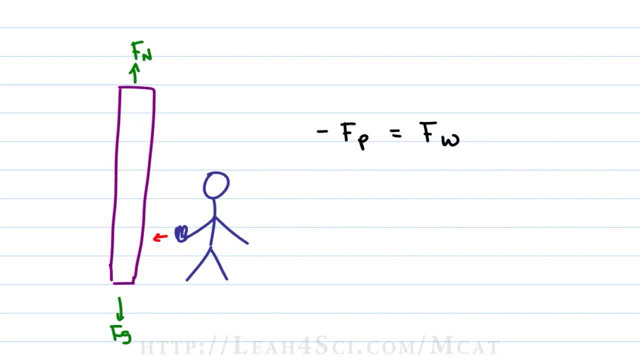 of the person by the foul, the way of layer of electric energy by the wall, Assuming the wall is capable of. with similar rate of power to the wall, You're likely shifting the force from the end of the balloon machines into the wall, nominally, assuming the wall is capable of withstanding that force. the wall simply increases its. 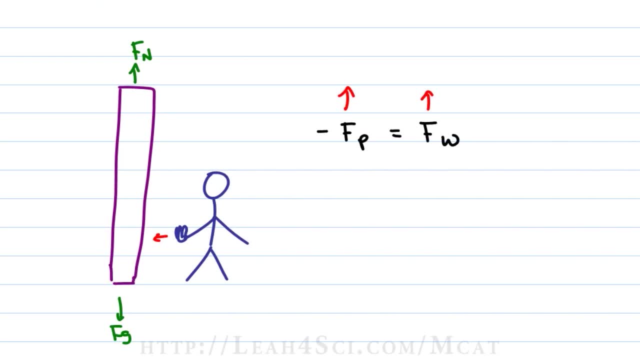 opposing force to make sure that it matches the exact force of your body slamming into it. And once again, the wall is at equilibrium. it doesn't move Now, assuming you're very strong and your body slam has more force than the wall is capable of preventing the wall. 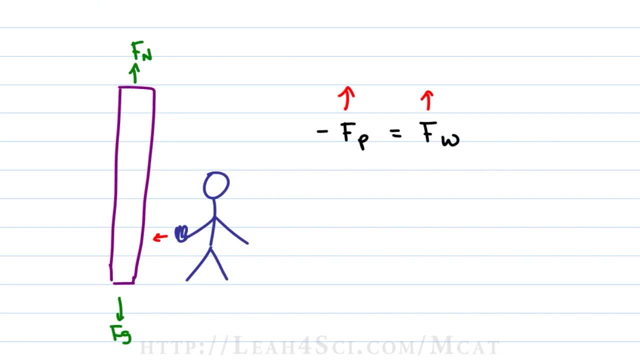 will topple over. This is a concept you definitely want to keep in mind once we tackle static and kinetic friction. Now let's end with Newton's Laws and start tackling the individual forces, including equations and calculations. You can find the entire series along with 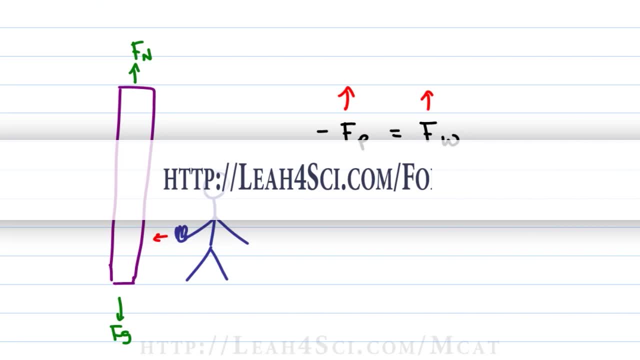 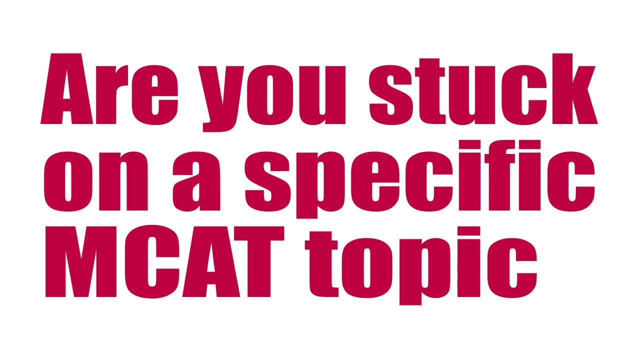 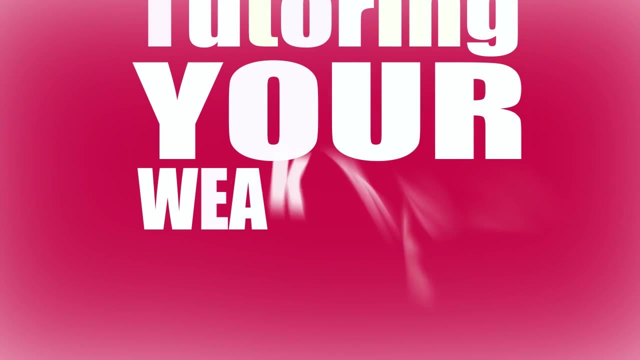 my Forces Cheat Sheet and Practice Problems by visiting my website: leah4scicom/forces. Are you stuck on a specific MCAT topic? I offer private online tutoring where I focus on your needs to strengthen your individual weaknesses. Tutoring details can be found.